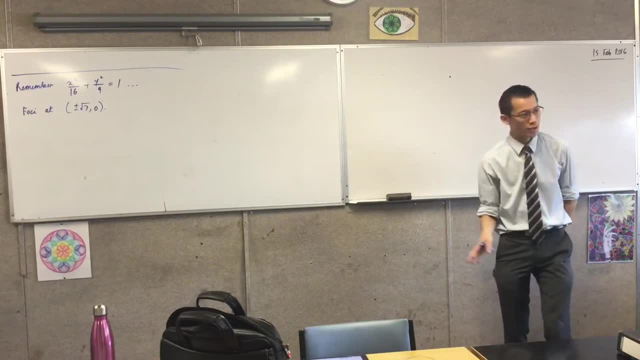 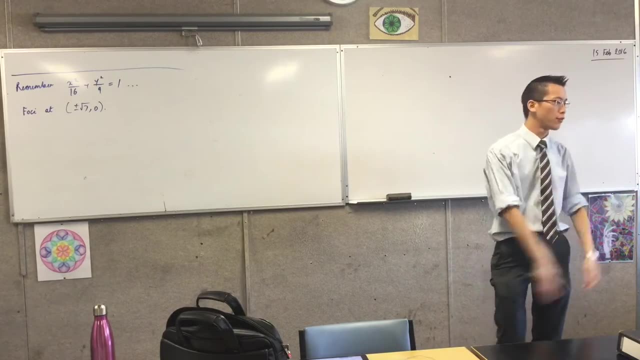 For a couple of reasons I'm not going to do that. first off, If I just deal with actual numbers, a lot of stuff will simplify out and the algebra will not be too involved. We'll have a look at the full algebraic proof a little bit later. 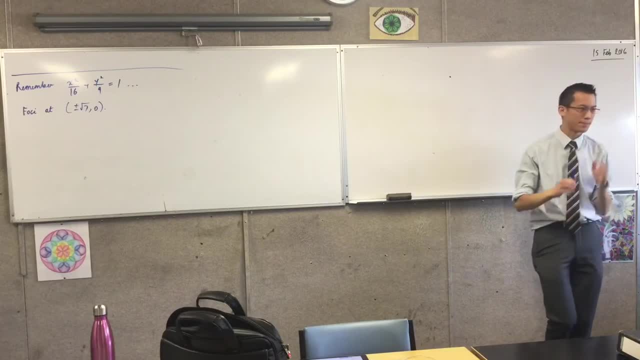 I'll show you how to do that. I'll show you how to do that. I'll show it to you. It's all written in fancy colors and what have you. But I think it's a bit confusing as to why you would do that before you see what I'm going to show you. 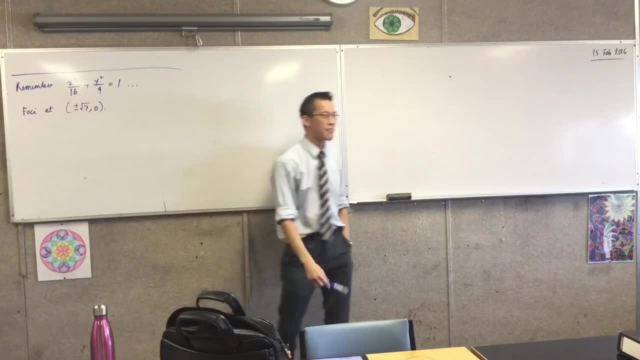 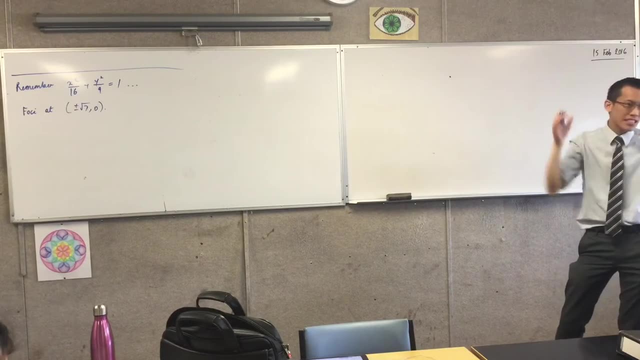 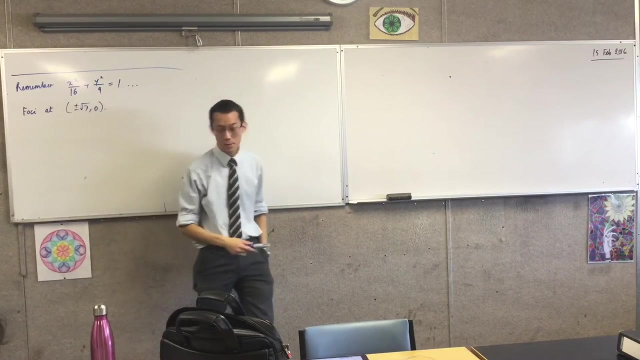 So let's call back to this ellipse. You know how I have my favorite quadratic. This is the equivalent for the ellipse. This is my favorite ellipse, So I keep on coming back to this because it has relatively simple numbers. Now we actually determined that the foci of this ellipse are plus or minus root 7 comma 0. 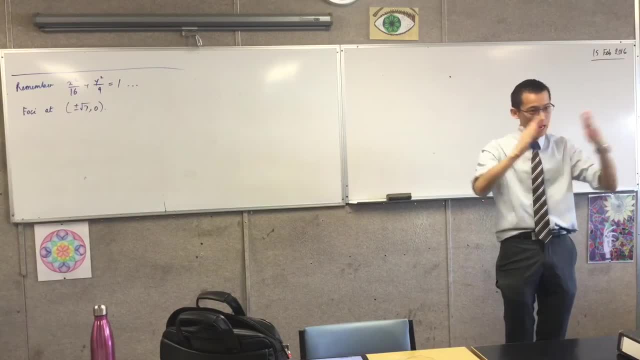 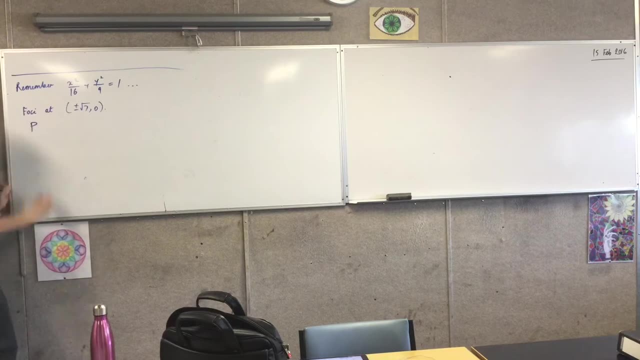 So it's. It's on the major axis, being horizontally, so I've gone out that far. okay, Now, noticing that, like thinking in terms of the locus right, You've got a whole bunch of points P, where they're according to X and Y, such that the distances to here, to these points, will always be some proportion of the distance to the directrix, or the directrice, I should say. 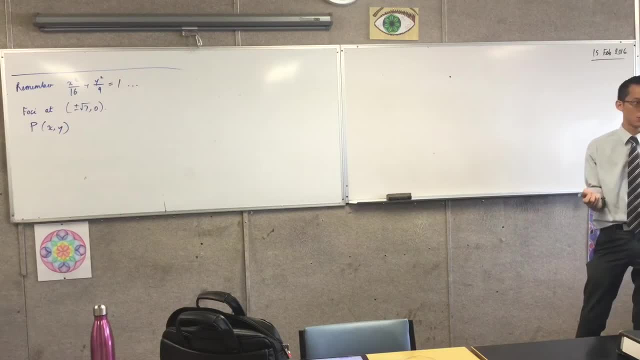 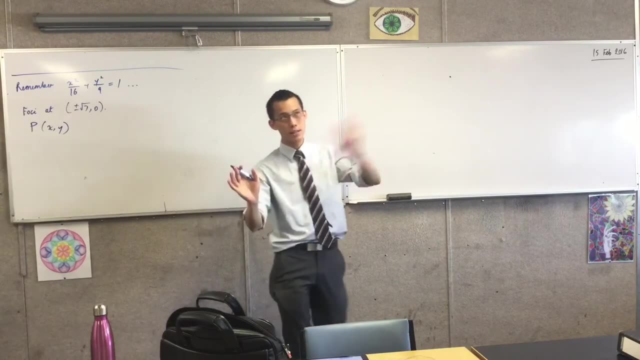 That's all fine. I want to do something a little bit unusual and less sort of obvious, which is to say: You know how there's two points, Two foci, right, And we said: well, you've got one, it's symmetrical, so you get another one. 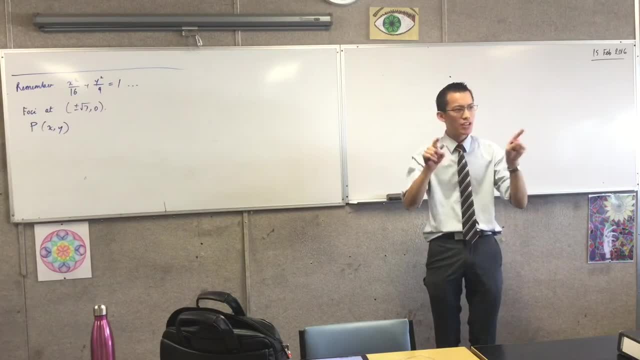 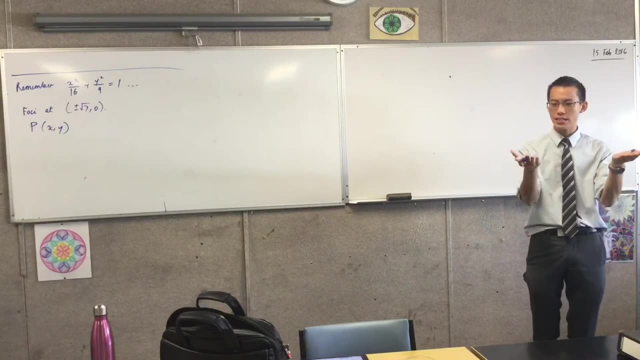 It's kind of like it's just there, right. My question is, though: do they have more of a relationship to each other? The Whispering Gallery is where we started at the very beginning of Coddick's. It kind of suggests that actually, the foci are related to each other, not just there by accident. 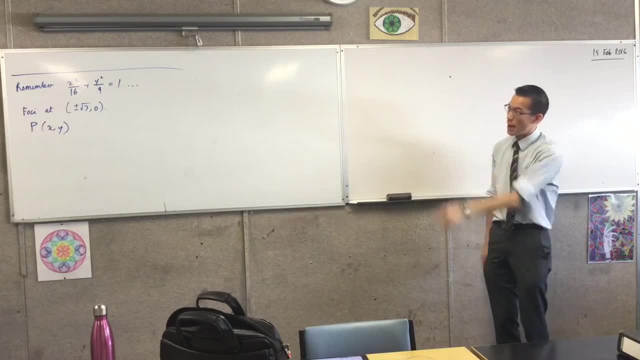 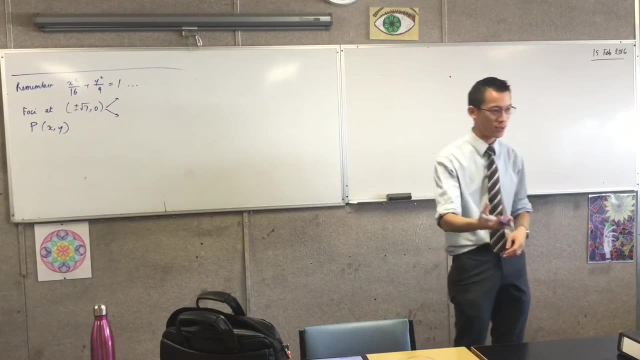 So I'm going to try and demonstrate the relationship between them by having a look at the foci as two different things. So you might remember we used to on the parabola. call them S, like that's the focus. 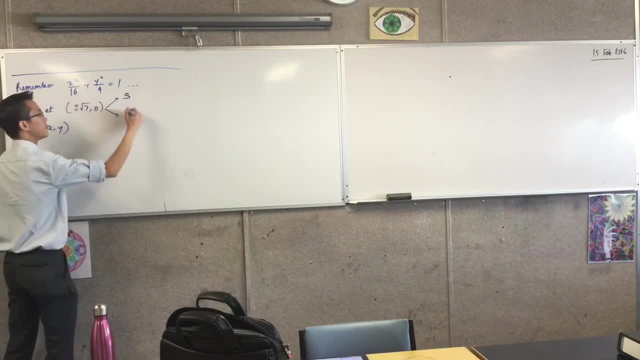 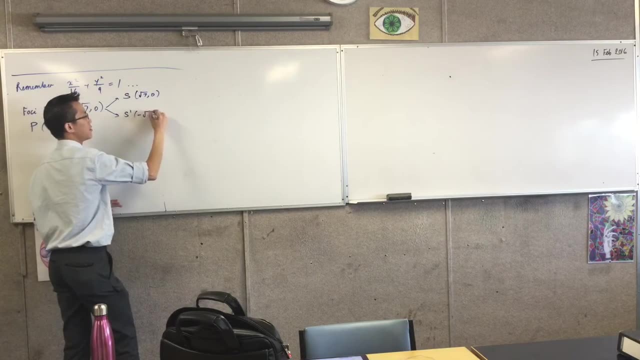 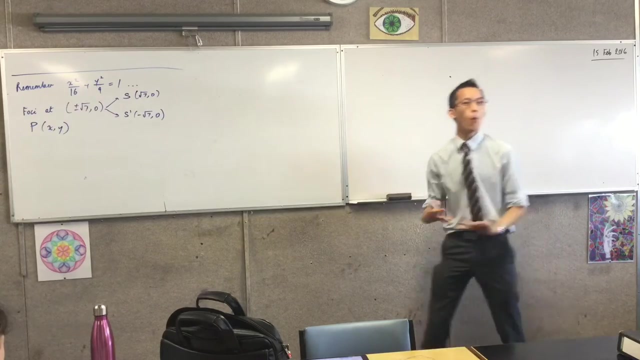 So, being that there are two, I'm going to call them S and S'. Now, if I designate what is the positive one, what is the negative one, I can start to do some work with this right. So, in particular, I am interested in, generally speaking, what is the distance from my point to the focus? 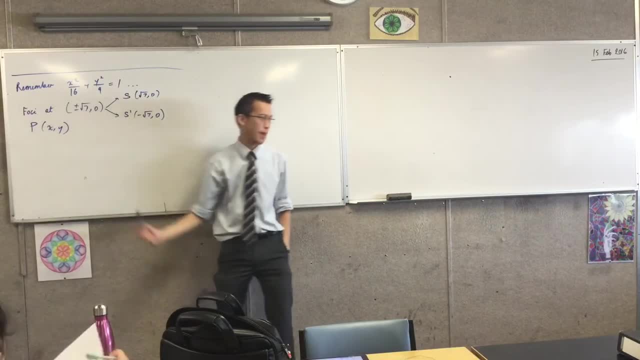 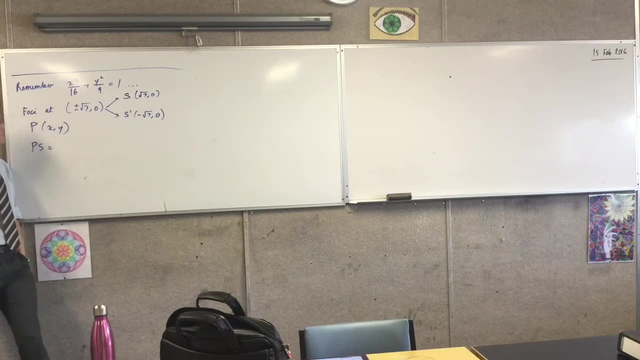 So when I say generally, I mean for any x-y pair, that's on the locus, okay. So how do I work out this distance? S It's just two points, right? Here's a point, here's a pair of coordinates and here's another one. 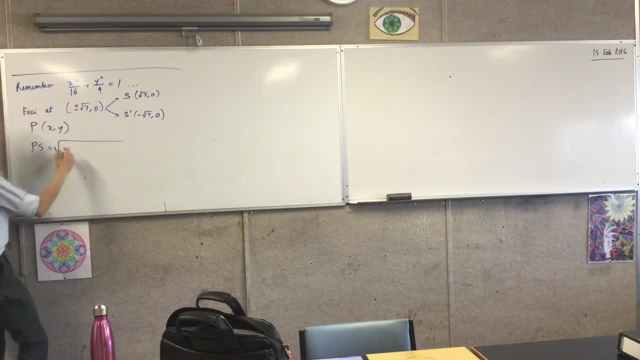 So let's just give this a crack, right? This is going to be the square root of: and I've got x2 minus x1 squared and then y2 minus y1 squared. You okay with that? Nothing too dramatic there. 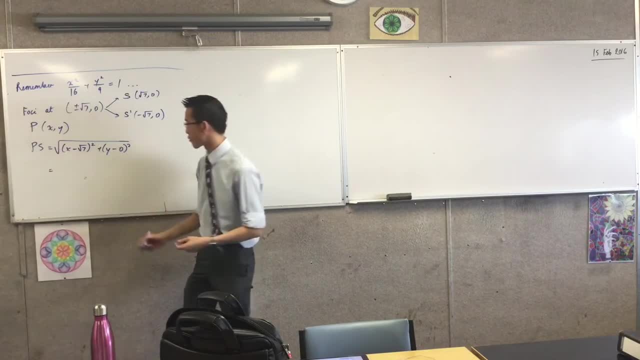 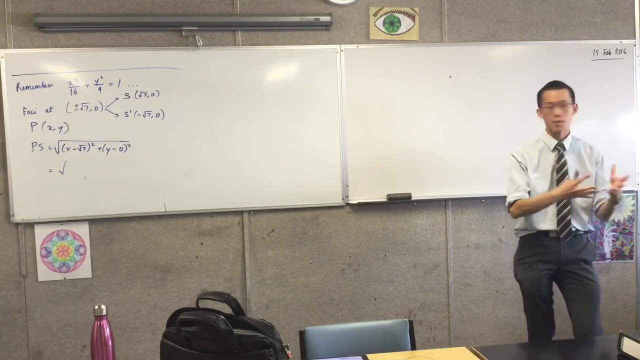 Now I can simplify this a little bit, right? I mean, I know that there's going to be some stuff. I know there's going to be some stuff that can simplify here, because, even though I've got x2 and y2 at the moment underneath the square root, 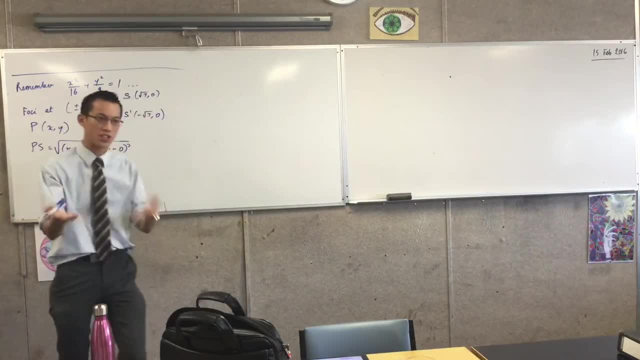 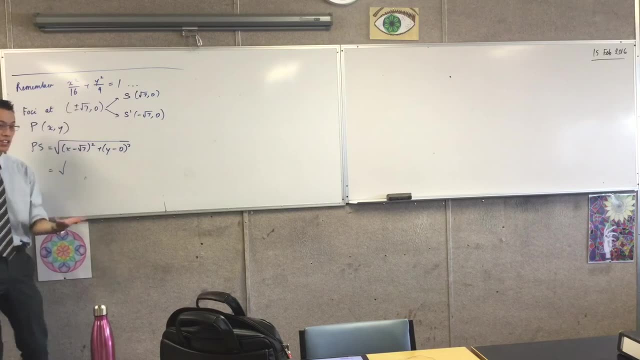 x2 and y2 are kind of interchangeable, not like just a straight swap. But this equation up here tells me there's a relationship between x and y. okay, So that suggests to me I should be able to eliminate one of these variables out. 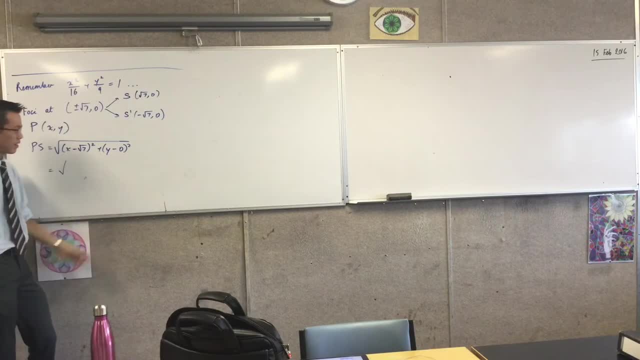 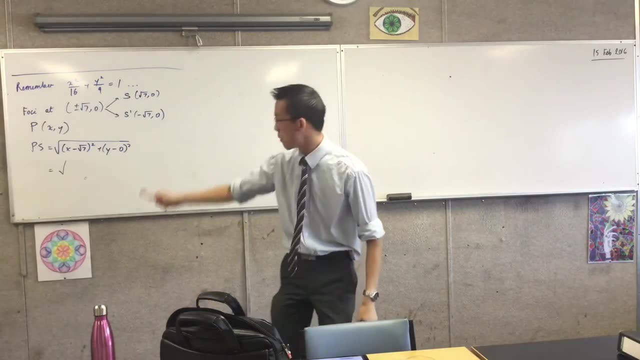 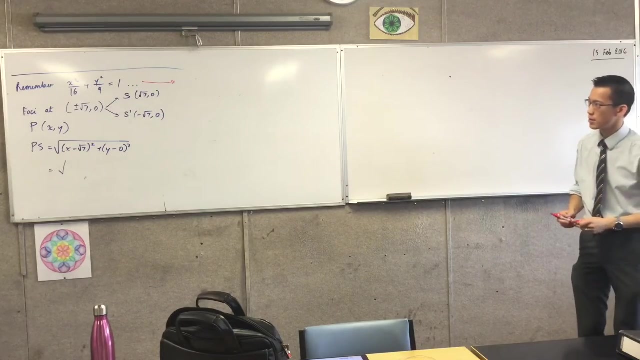 Now I can eliminate x2 out, or I can eliminate y2 out Just because y2 is on its own. I think that would be easier to do, okay, So have a look at this line for a second Before we march on with our work. if I were to make y squared, the subject of that equation in the ellipse, what would I get? 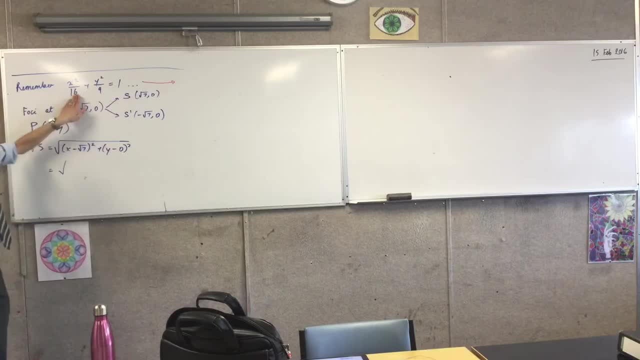 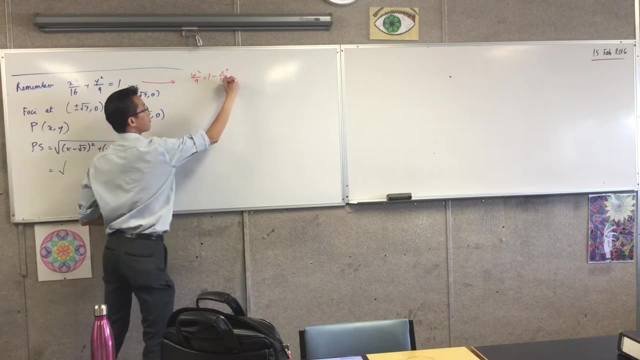 What should I do? What should I do? first, Take the x squared on the 16th Yep. I'll move that term over. That gives me this Yep, and then I'm just going to multiply through, aren't I? 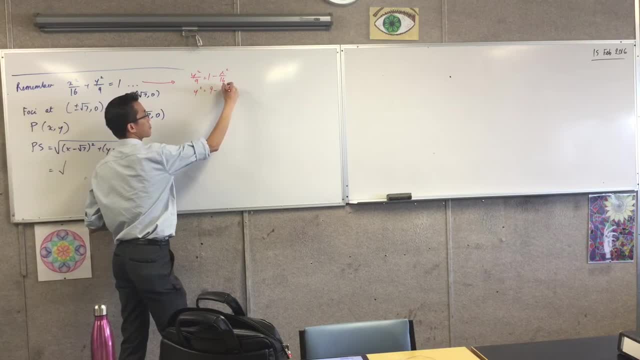 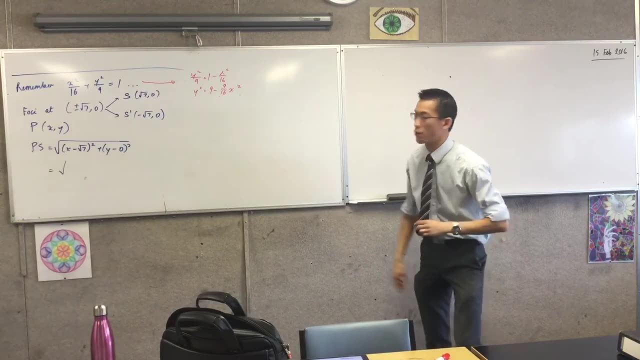 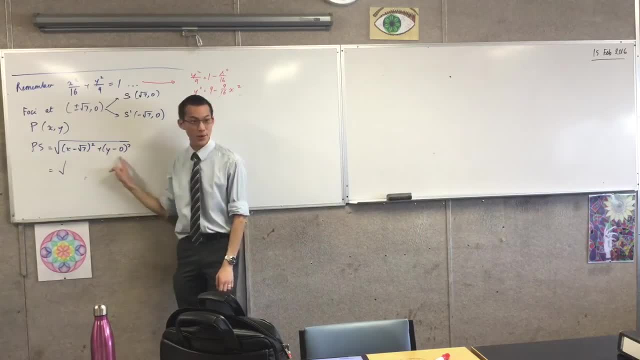 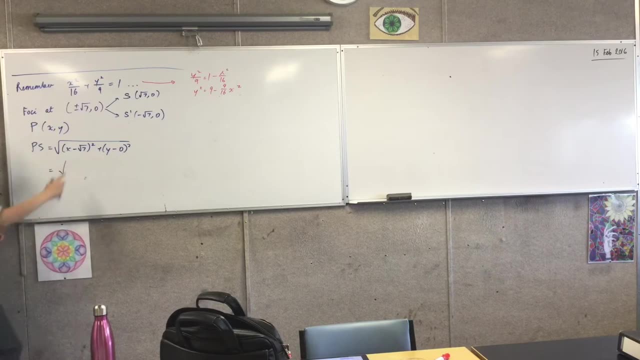 me everything in terms of x squared, So I'm hoping- my fingers are crossing- that there's going to be some collection of like terms and things can simplify out in some way. Okay, So let's have a crack at expanding this. 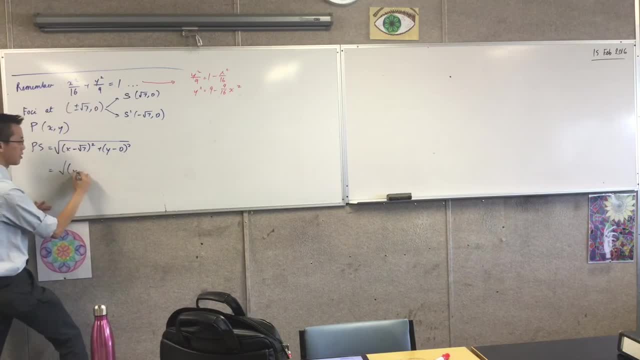 This part here is going to be- I mean, it's just going to expand a perfect square, So it'll be x squared minus the sub root of 7x plus 7.. Good, Good. And then, instead of writing y squared here, I'm going to substitute that for x squared. 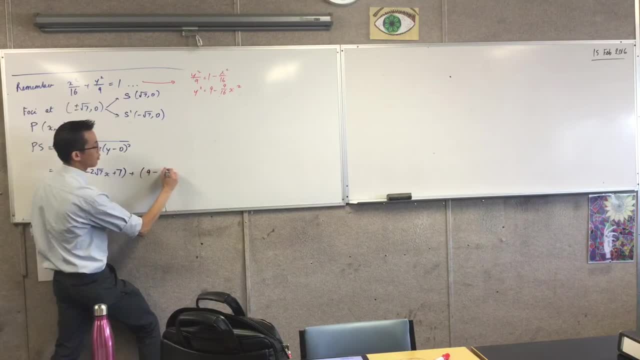 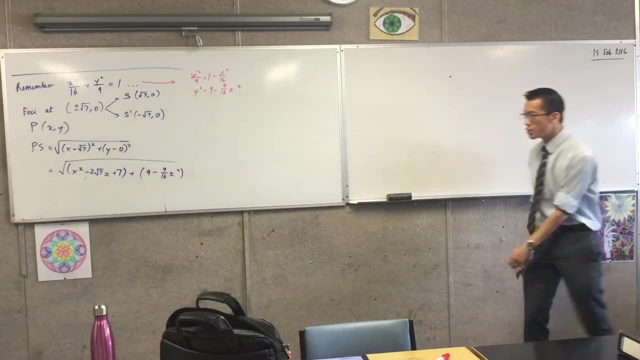 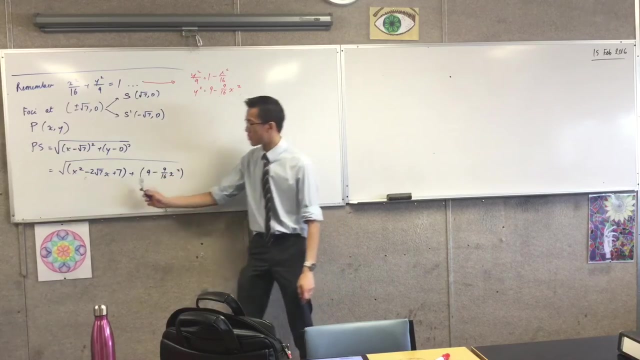 This guy. Okay, So I'm getting 9. take away this many x squared And that's all underneath the square root. Okay, So you can see, as I was hoping for, not just 1 but 2.. These two terms are both going to collapse into the terms that I got from extending this. 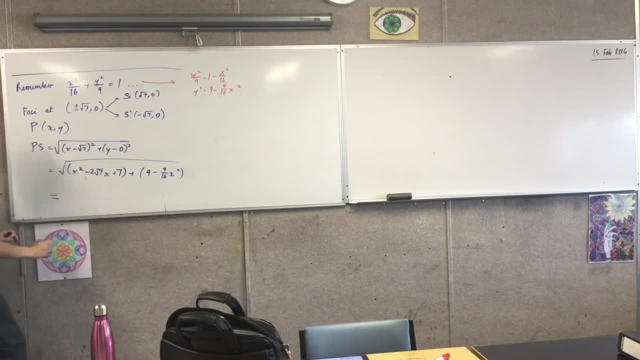 square Right, So let's collect some things together. I've got the square root of: okay, how many x squared terms do I have left? 7,, 9,, 6.. Yeah, it's one of them here. 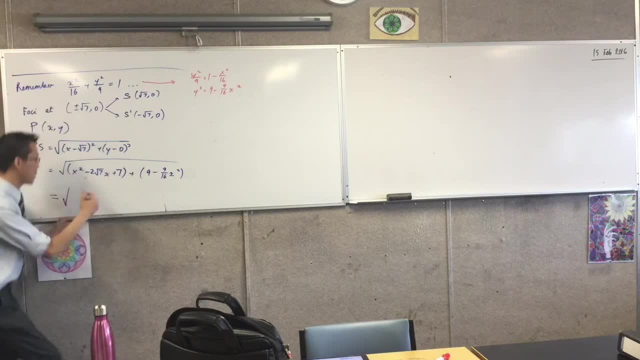 And I take away 9 sixteenths of 1 here. So that leaves me with 7 sixteenths of 1 here. You okay with that? What about the x term? Does anything happen to that? It just stays good, doesn't it? 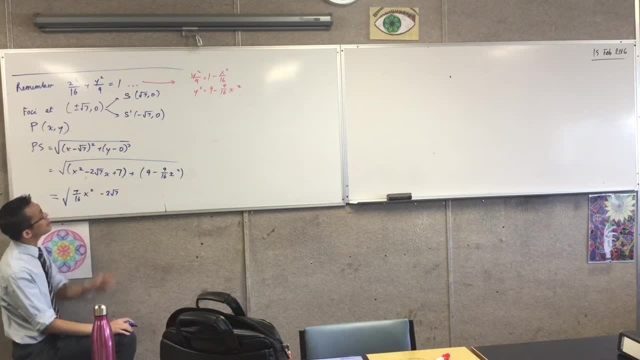 2 root 7. And then here I've got plus 7 plus 9. Plus 16.. Does that look okay? Happy so far. Minus 2 root 7x: Sorry, yes, that's an x. 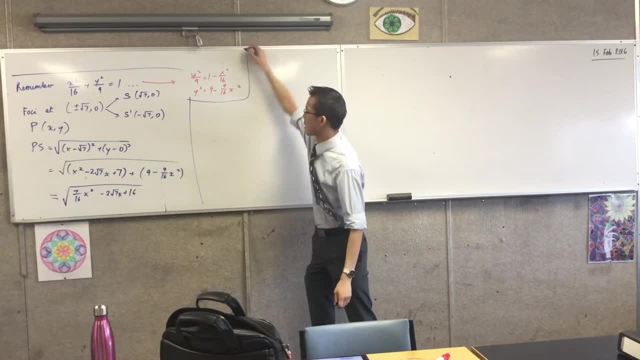 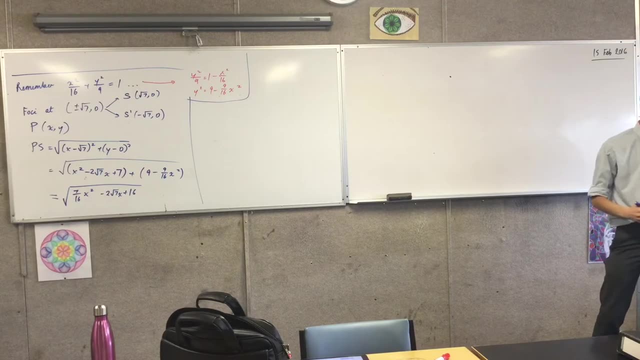 Thank you, Very good, Okay, so let's just move that guy on. Okay, now look at that, Stare at it hard. This is, believe it or not, as easy as it gets. It's got the least number of thirds I can possibly put into it, and at least certainly 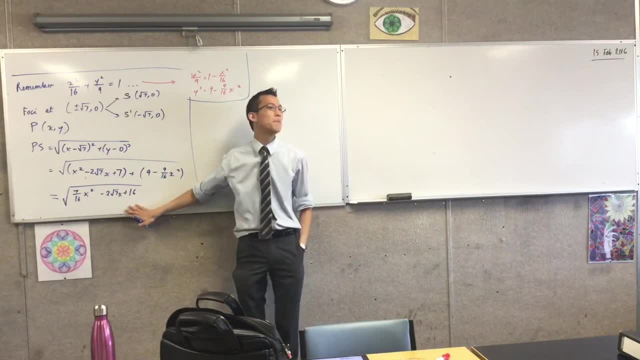 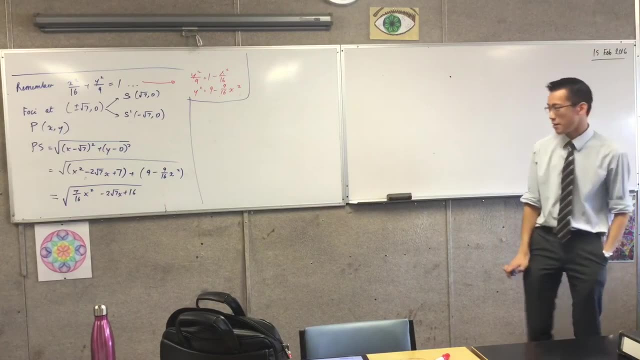 the least amount of algebra that I can put into it, even though it is not at all immediately obvious. This guy here is a perfect square. Not an obvious perfect square. Have a look though. Okay, I can do the easy part of it first. 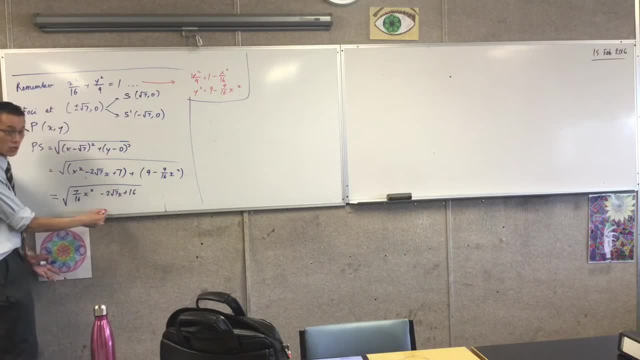 You're expecting like an a squared plus or minus. You're expecting an a and a b squared right. So what's the b squared going to be? It's 4 squared right. So this is plus 4 squared right. 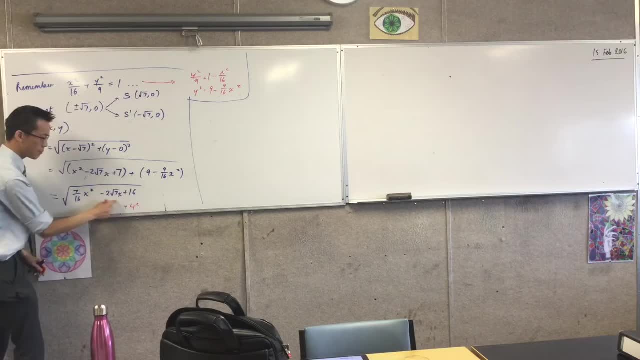 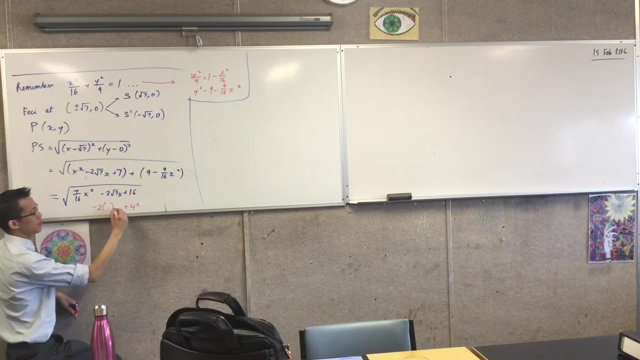 Yep. So if that's what b squared is, this should be. since there's a reason, I guess this is minus 2ab. yes, Minus 2 times something times 4.. So what's a? What would give me minus 2 times something times 4?? 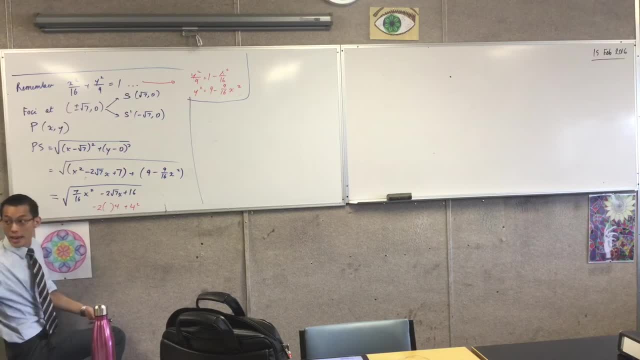 Yeah, good, Because I've got 8 here and there's a 2 there. it looks like I have to divide by 4.. That'll give me the. I'll end up with the 2 there, right? It'll exactly cancel with that. 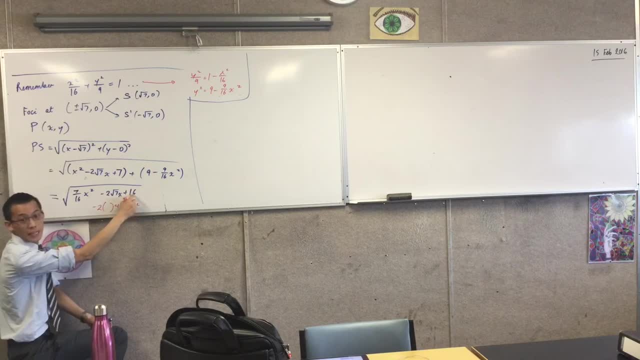 And you've got a root 7 and an x there as well, and they can't come from here. obviously There are no thirds here and there are no x's, so it must come from here. Root 7: on what did I just say? 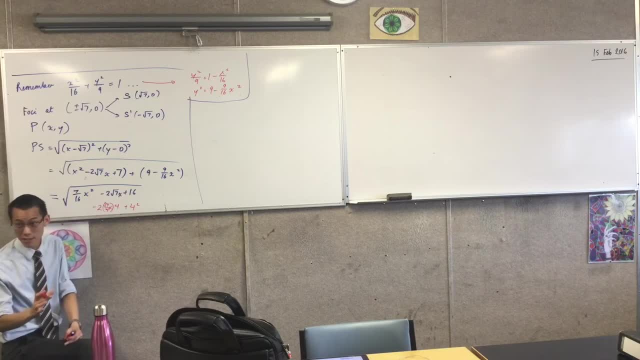 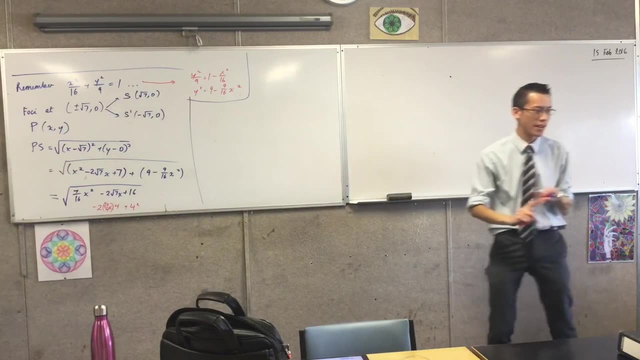 4x. Do you agree with that? It's a bit messy, right, But trust me, this is as few thirds as you can get For what it's worth. So if a and b are whole numbers, e will be a third, and if e is a whole number, then 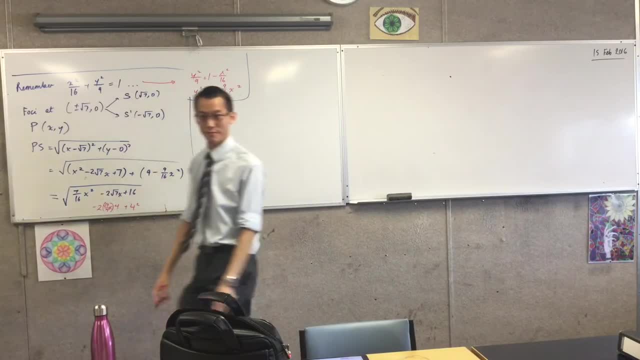 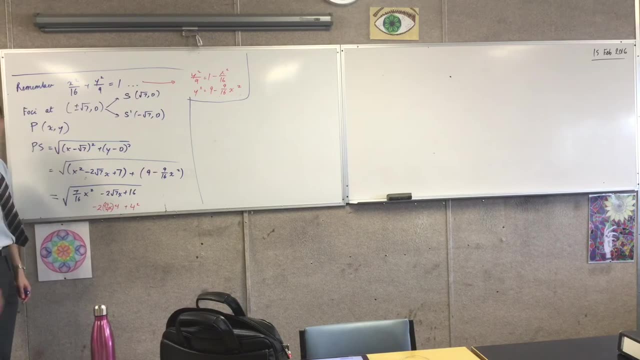 a and b will be thirds. Okay, yep. Is it a coincidence that 7 on 16 equals to e squared and root 7 is 2 times the x-coordinate of the bronchi. No, it is not coincidental at all. 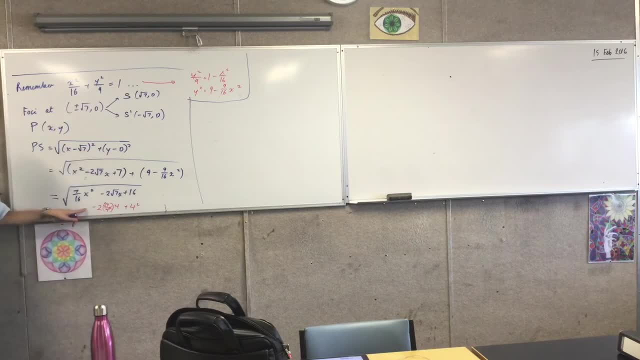 So I will get to the algebraic one in a minute, but let's just finish this off here. I've just identified this is the a, and you can see it fits with this, doesn't it? This is my a, squared. 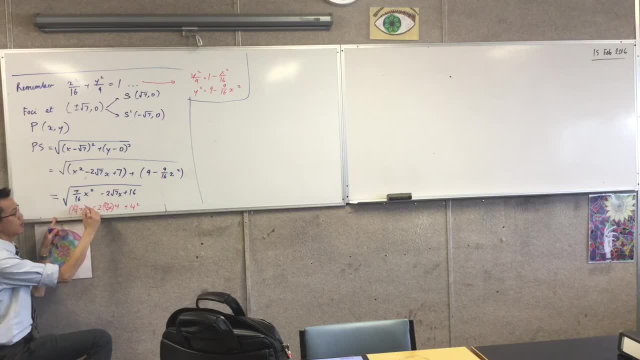 So this looks like to me it's root 7.. Root 7 on 4x, all squared. Are you okay with that? And that's all taking the square root. So now the factorization for the perfect square is a little more obvious. 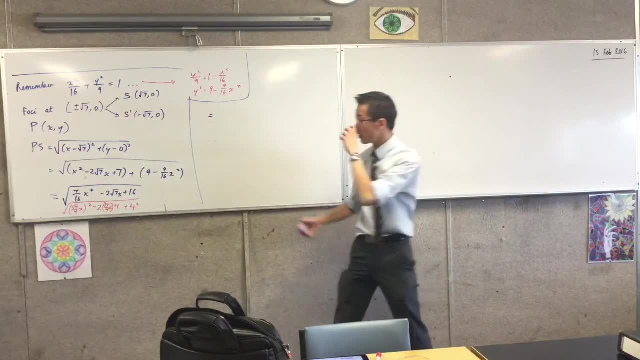 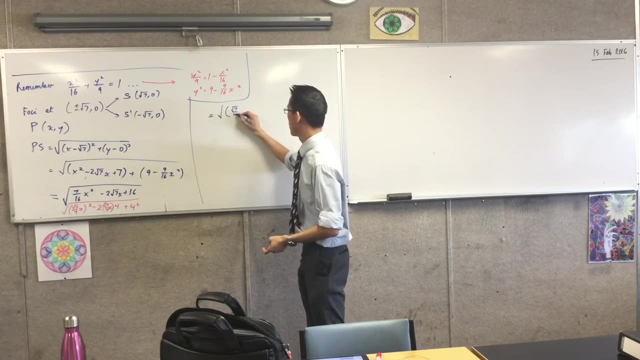 So what am I going to get? This is the square root of a square, the square root of what's actually being squared. Root 7 on 4, x. take away 4, because I've got the subtraction in the middle. 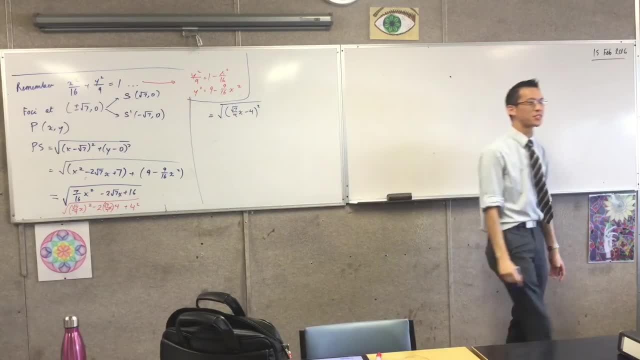 Looking good. That's squared and that's the square root, And hopefully I've schooled you enough to know that when you take the square root of a number, the square root of the square root of a number, you don't just get the number. 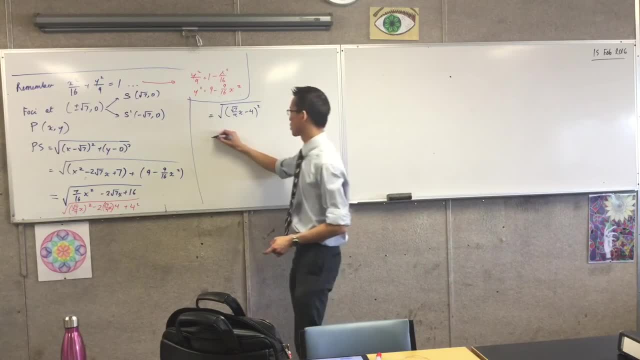 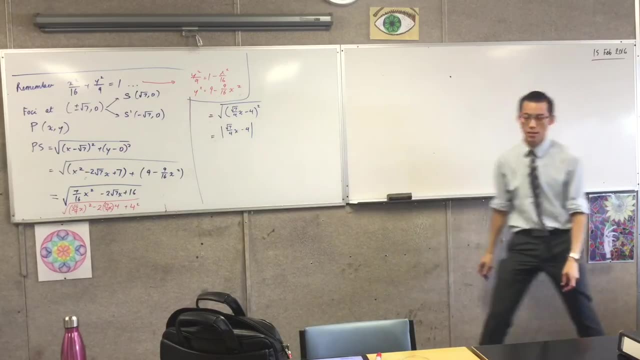 back. What do you get? You get the absolute value of that number. So it looks to me I'm getting this, Is that okay? Okay, now, for reasons that will become clear in a minute, I'm actually going to turn this. 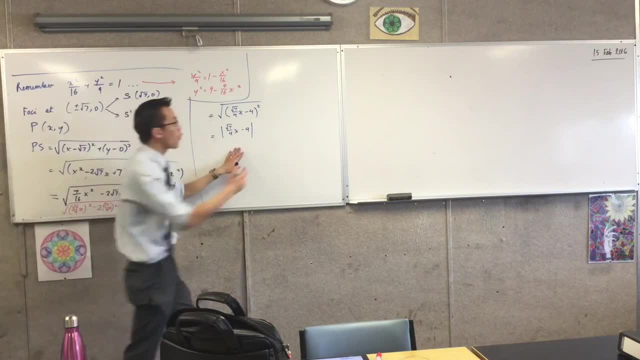 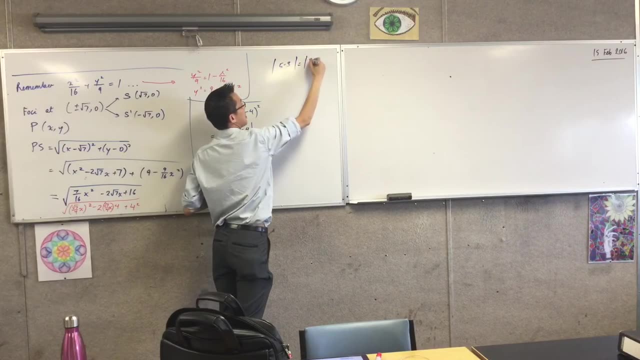 around, because do you agree, right, that the absolute value of, for instance, right 5, take away 3, don't tell me what the number is, just do it in your head. Do you see that this is the same as this? 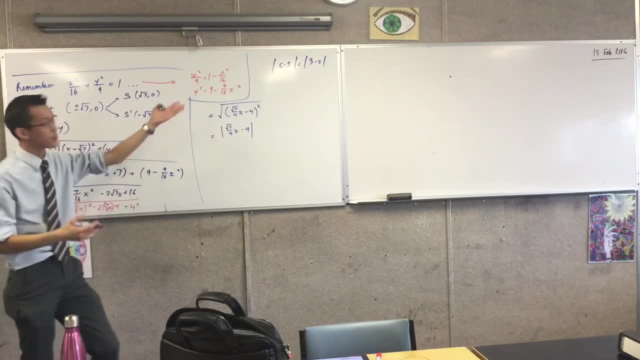 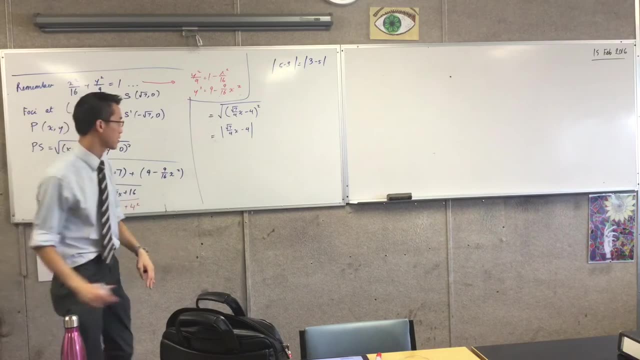 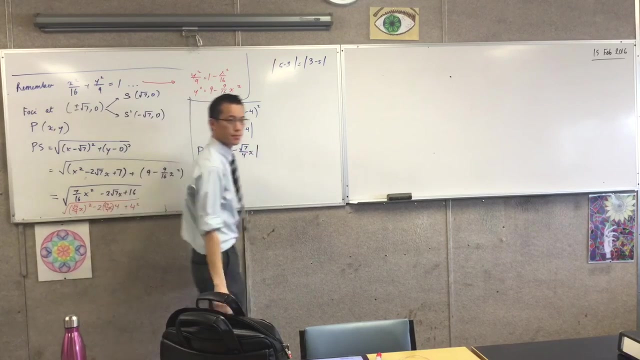 Right, Do you agree with that? Like, because it's taking the difference between the numbers inside the absolute value sign is a negative and the absolute value takes the negative out of the plan. right, Does that make sense? So I'm going to write it like this: 4 minus that's p s okay. 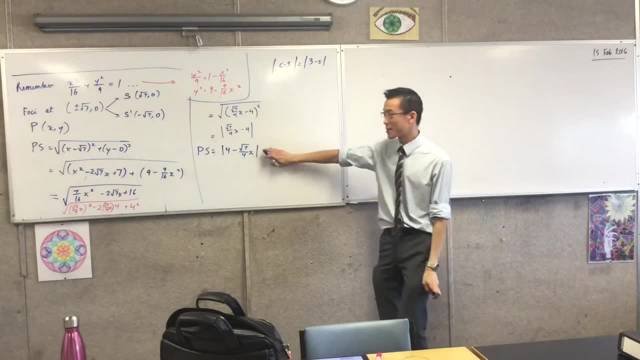 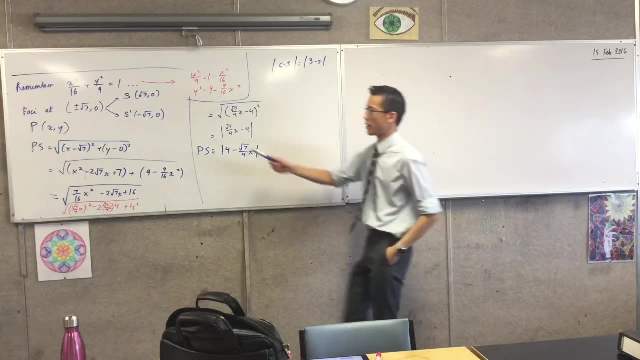 Now pause for a minute. That looks a whole lot simpler than what we started with. okay, I want you to look carefully at what will happen when I do it with the other focus. right, Have a look. What difference will it make? 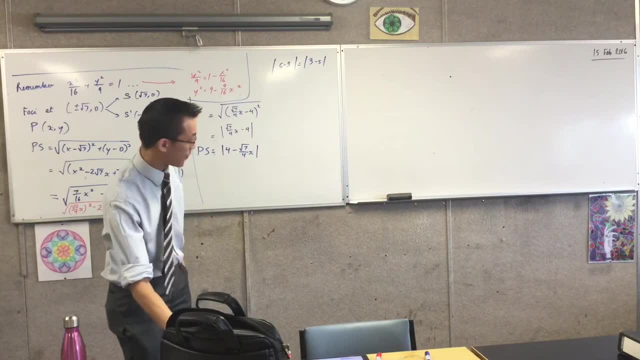 Nothing. 7 plus- Wait, what are you saying? Plus root 7.. It's very, very close, isn't it? Do you see? So, because everywhere I would have put a root 7, I'm going to put a minus root 7,, okay. 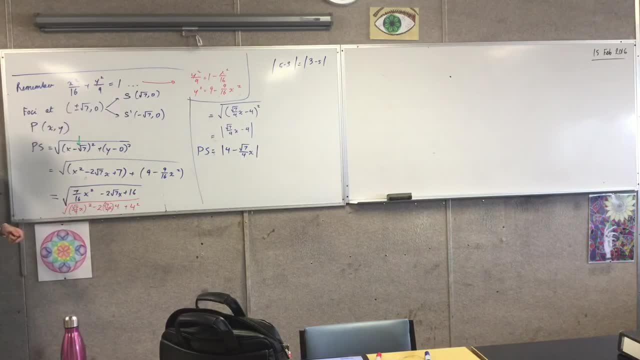 So in here, there's going to be a plus instead of a minus. That means, in here, instead of a plus, I'm going to get a minus. That doesn't affect with any of these, So that's still going to be here. 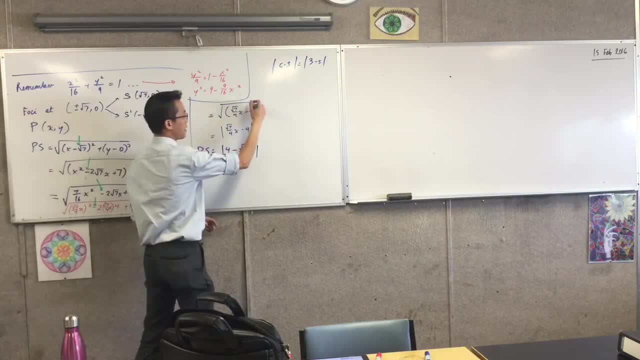 It's still going to be here. It's still going to be Now at this point. that's where I got my minus sign from. Do you notice that? So all the way through all these minus signs, they would have been pluses. 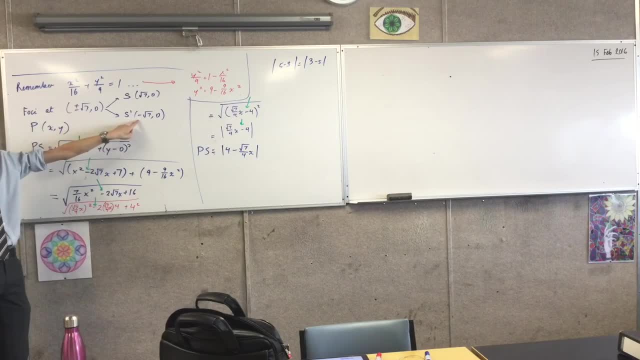 There's a double negative happening here, Yeah, so therefore, I mean you can do all the way through. but I'm just going to say similarly, by exactly the same logic, except with pluses instead of minuses, I'm going. 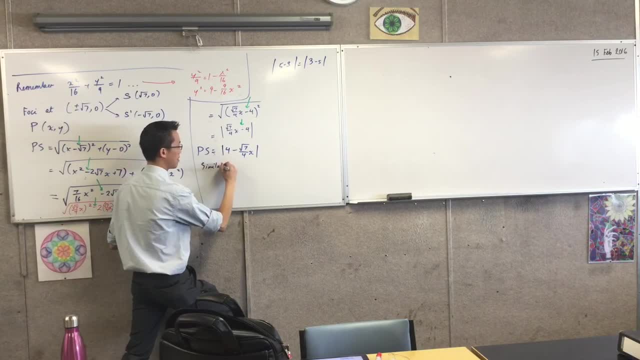 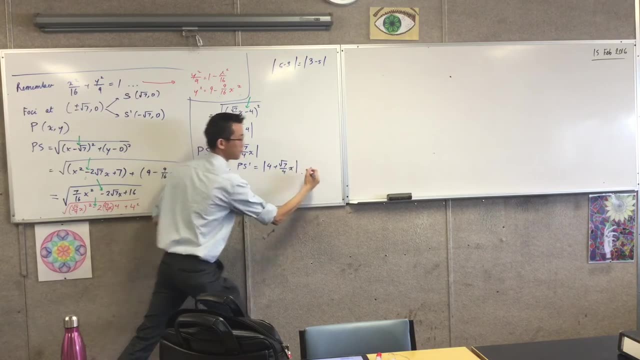 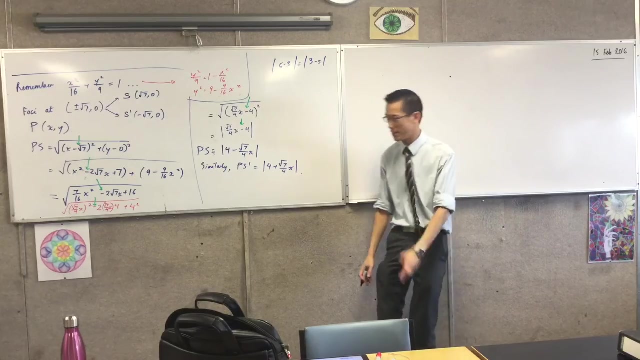 to say similarly: p s dash equals. I don't know, I've got to put it this way. I don't know. equals this guy? okay, now we are almost there. I know this doesn't seem particularly obvious that you would do this, but remember, I was trying to get a. 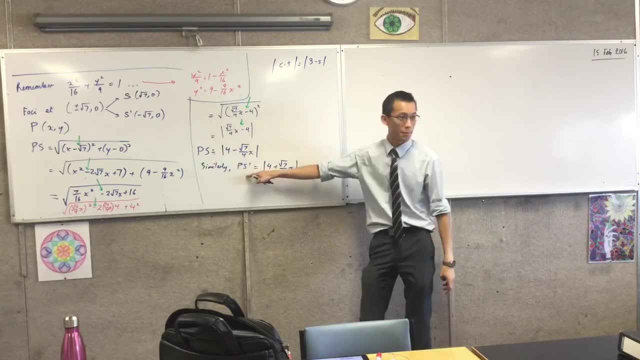 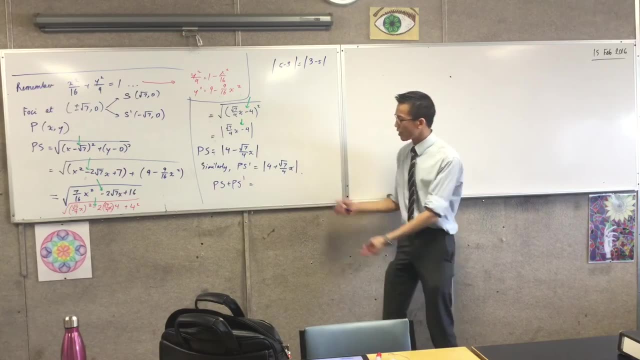 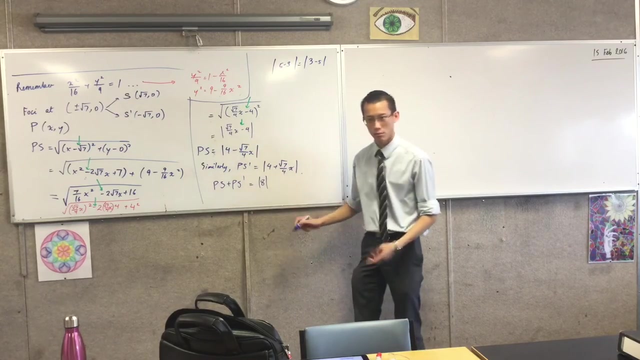 relationship between the distance to one focus and the distance to the other. right? well, you can see, if I just add them together like so right, can you see that there are two parts that cancel each other out? there's the negative there and the plus there, so I'm getting the absolute value of 8, which, of course, 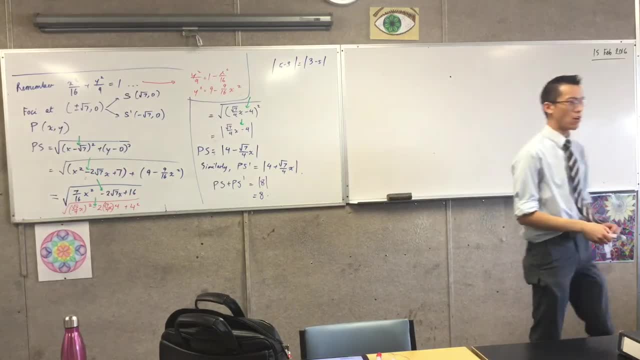 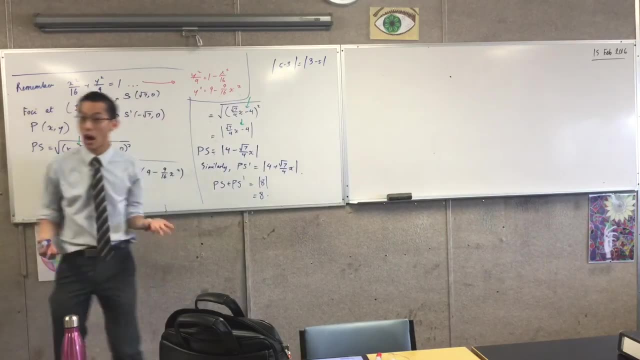 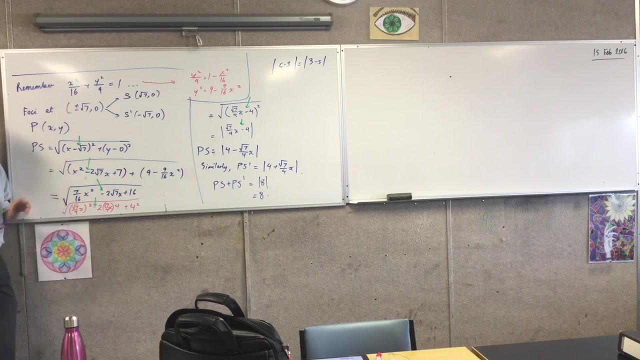 is just 8. now hold on a second. what have we just established? rewind all the way back to where we began, and what PS and PS- are? they are the distances to what. what are the distances between what? the distance between any point, and compared to one focus and then the other, mark that.